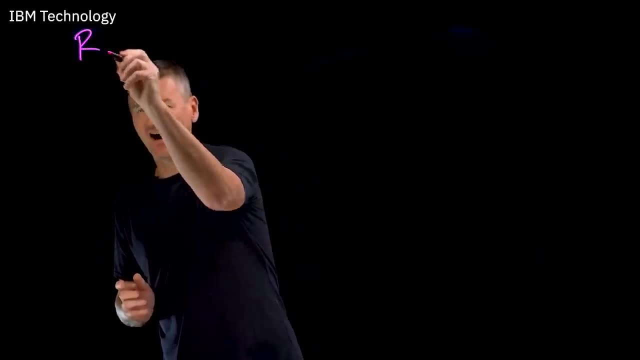 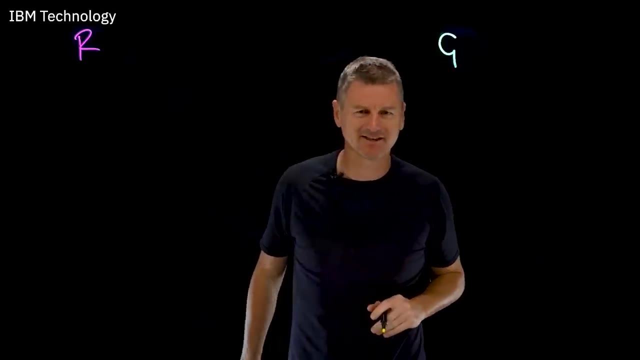 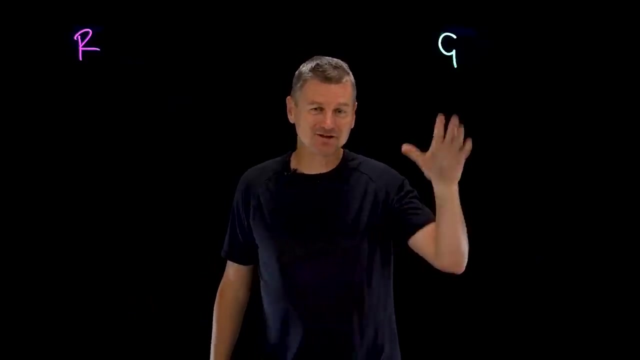 So I have these two colleagues. Let's call them R, and then we'll call the other one G, Just using initials here to protect their identities. Now, R is rather talkative: They tell you everything they know, whether you want to hear it or not. G, on the other hand, is much more. 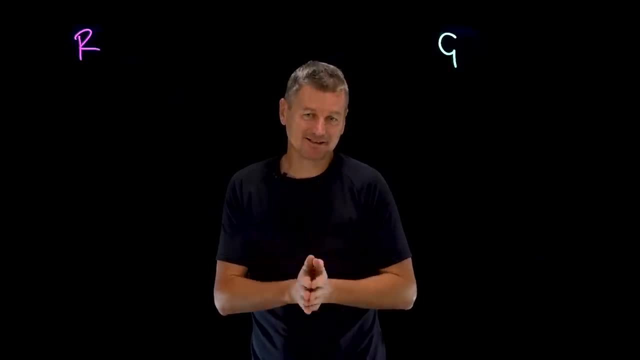 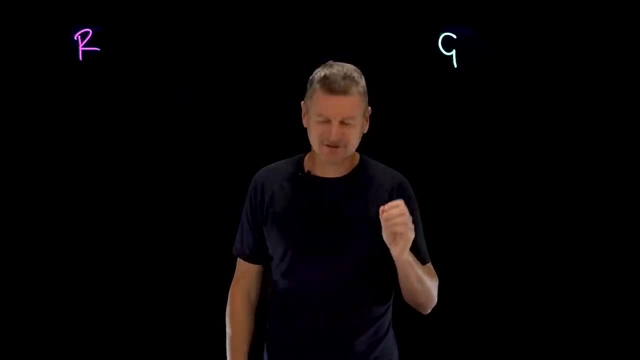 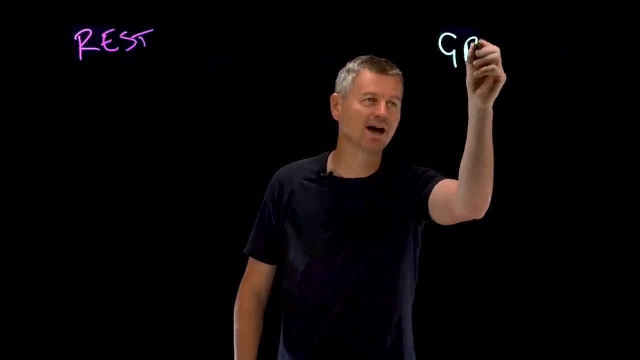 reserved. They share the information that's absolutely necessary, but no more. But they're always willing to share more if I do ask. And look, this is one way that we can think of the differences between REST, that's the R, and GraphQL, that's the G. REST can be a bit of a. 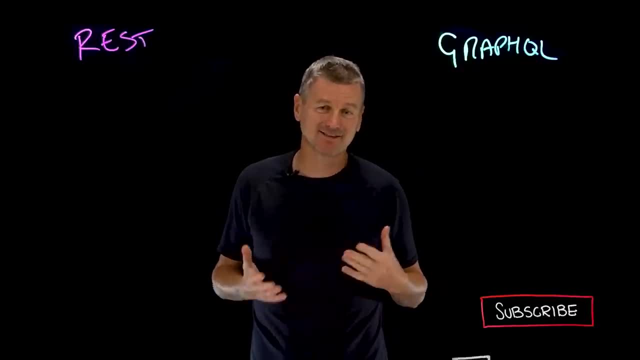 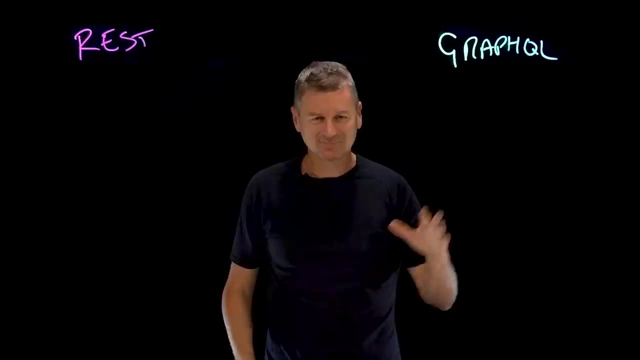 know-it-all. You have to be specific in your requests and sift through all the data that's returned. With GraphQL, you can be precise and only retrieve the data you need. It's said that GraphQL prioritizes giving clients exactly the data they request, and 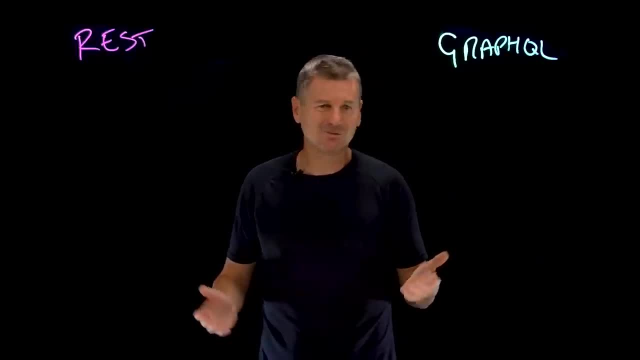 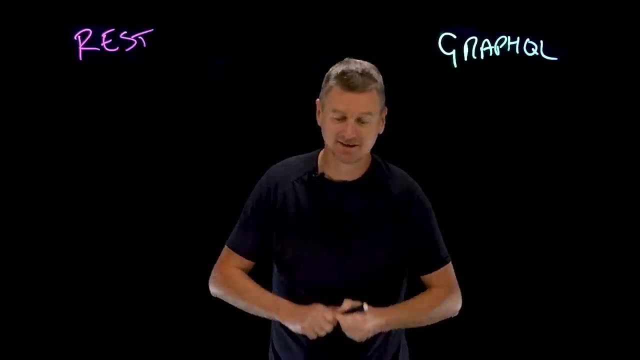 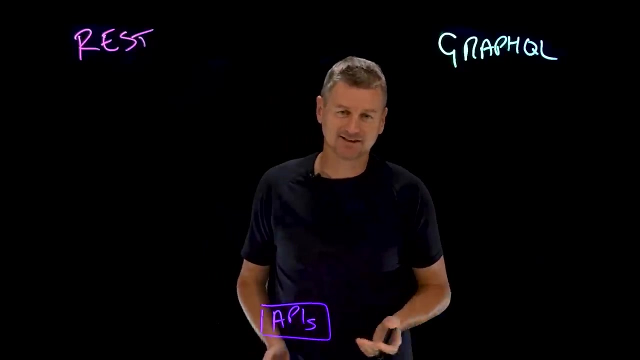 you can know more, But I'm getting ahead of myself here. What clients? What do these technologies do? Well, both REST and GraphQL are used to build something called APIs, or Application Programming Interfaces, And those allow different applications to communicate with each other over the internet. 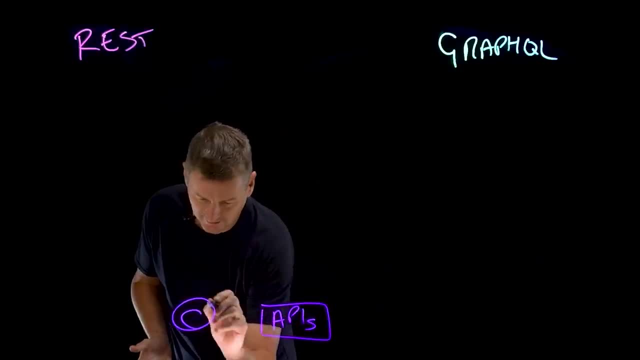 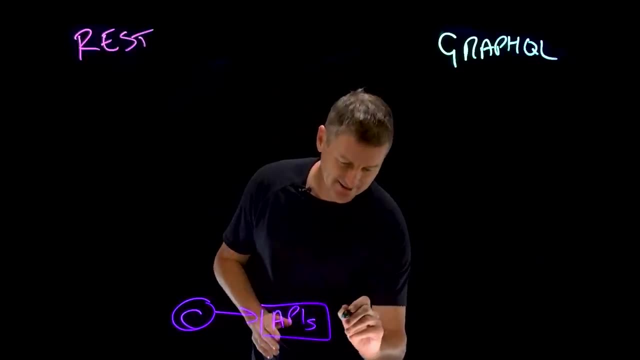 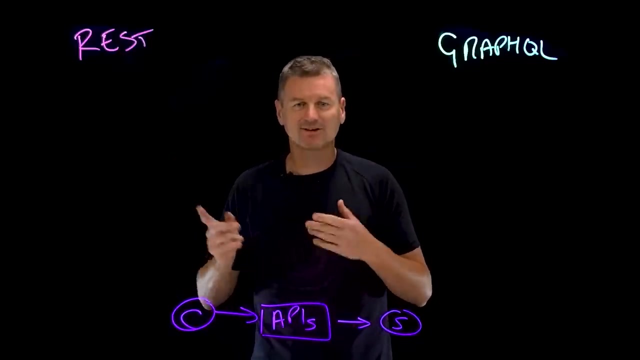 So an API takes requests from a client over here and that client can be like a web application Or a mobile app or something like that- And then it retrieves the necessary data from a server over here. Now, REST, or Representational State Transfer, and Graph Query Language are two different. 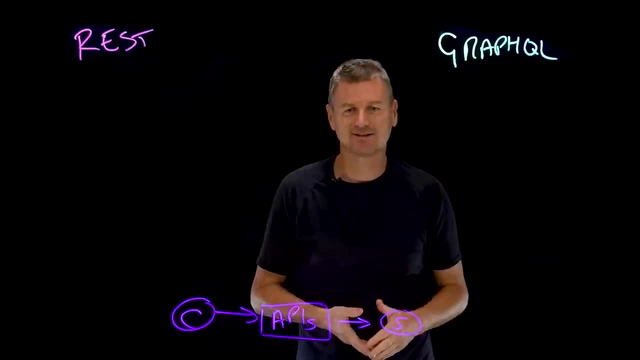 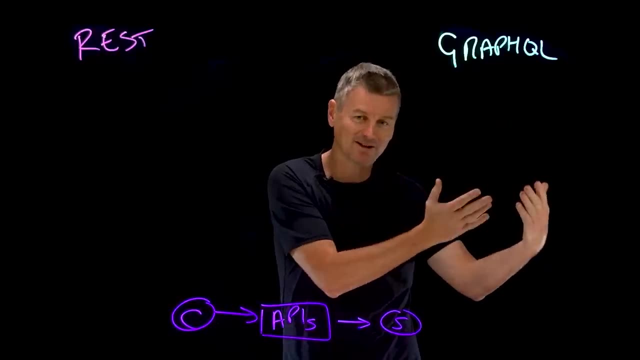 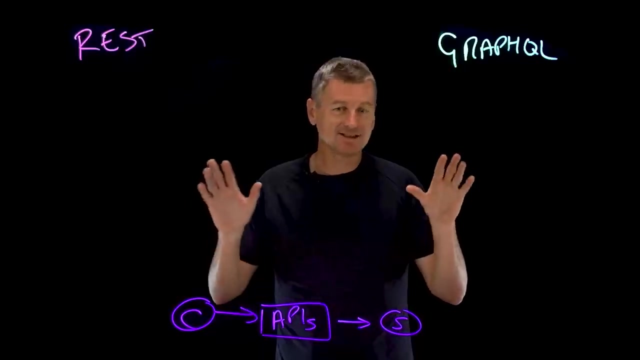 approaches to building APIs that have their own strengths and weaknesses. So REST is an architectural style that relies on HTTP requests to interact with resources, while GraphQL is a query language that allows clients to retrieve data from multiple data sources in a single API call. So let's define some terminology and we're going to start with GraphQL. 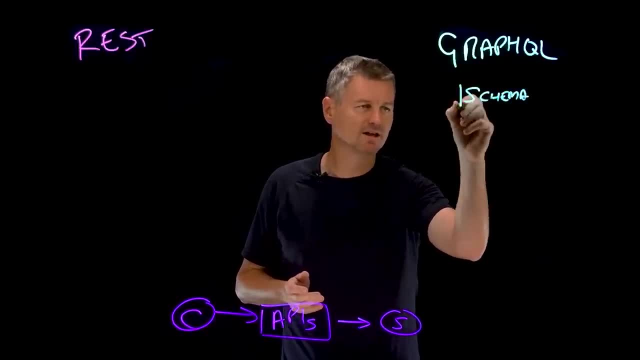 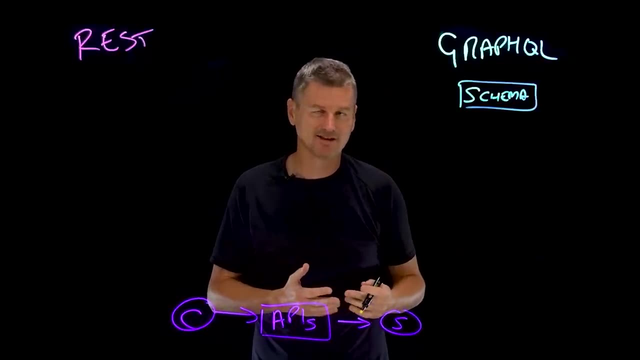 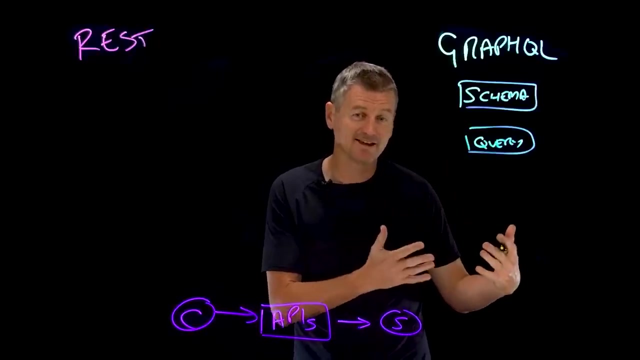 So in GraphQL we have something called a schema and this is the blueprint that defines all the possible data that clients can query through a service. Can I say query? Yeah, query, that's the next one. So a query is a request for data that follows the structure defined in a schema. That's. 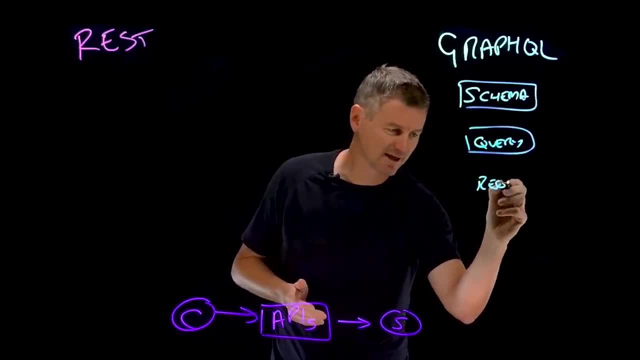 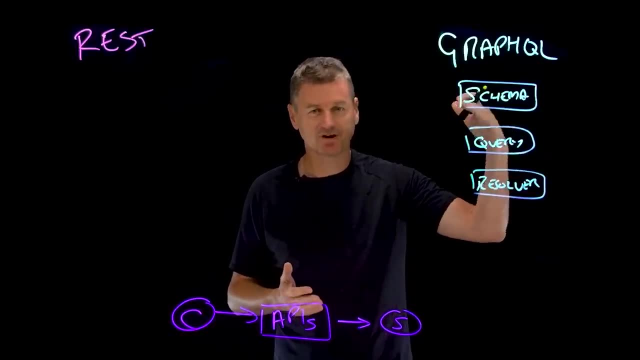 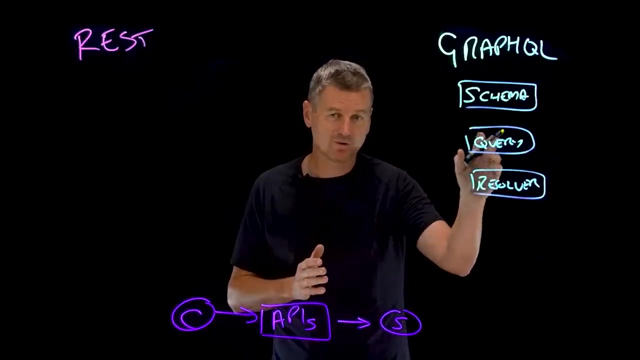 in the schema. Then we have something called a resolver, And the resolver is called to retrieve the data requested in the query, And this may involve fetching data from multiple data sources and assembling it into a response that matches the query structure. And then, lastly, we have mutations. 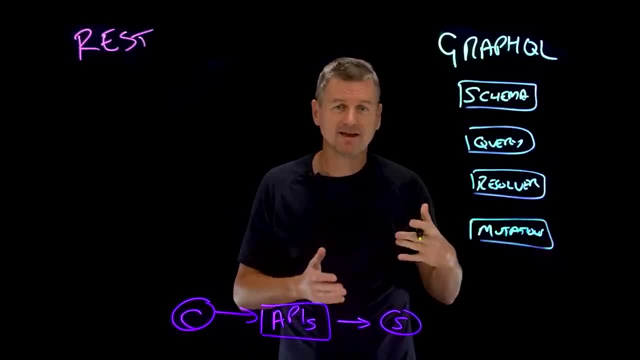 and mutations. Their job is to modify data on the server. So if we think of this in terms of the create, read, update and delete of the CRUD model, a query that would be equivalent to the read in a CRUD, and then all the others. 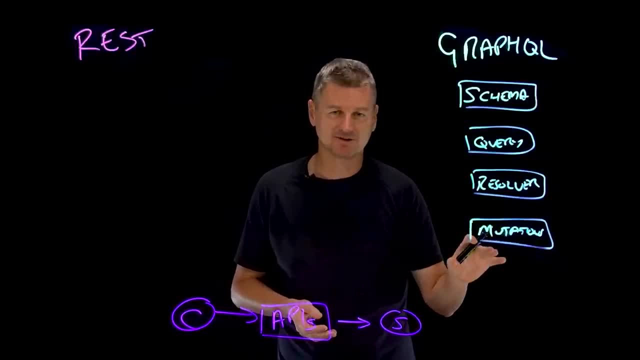 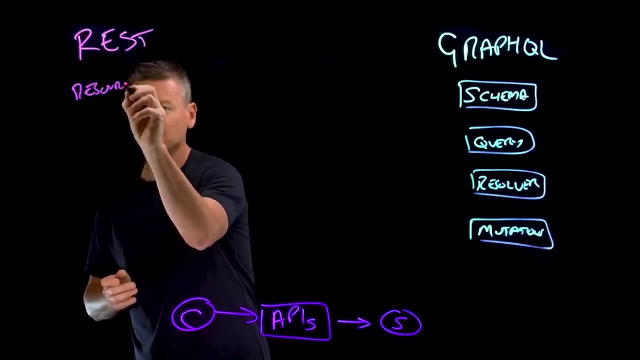 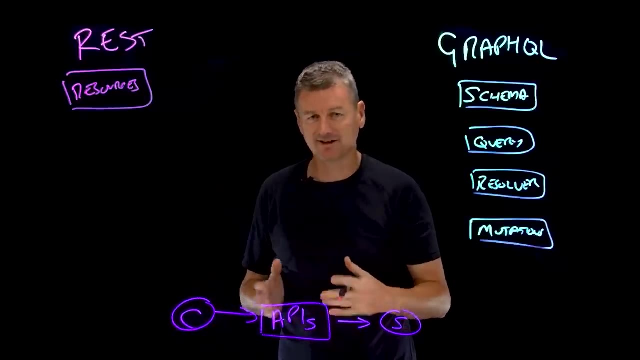 that create the update and the delete. they're handled by mutations, So that's GraphQL. If we take a look at REST, we consider resources in REST. So resources are really the fundamental concept in REST and each resource has a unique identifier called a. 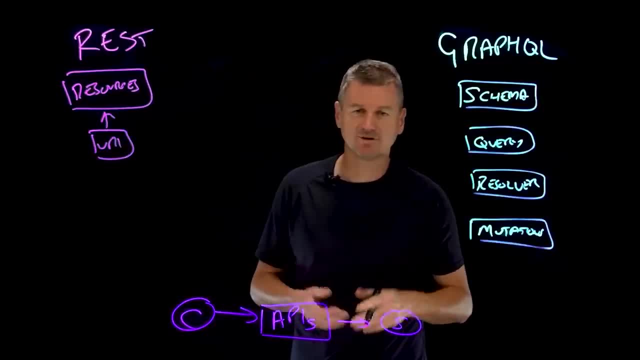 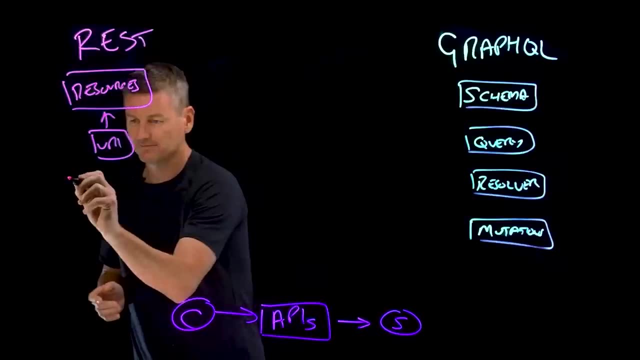 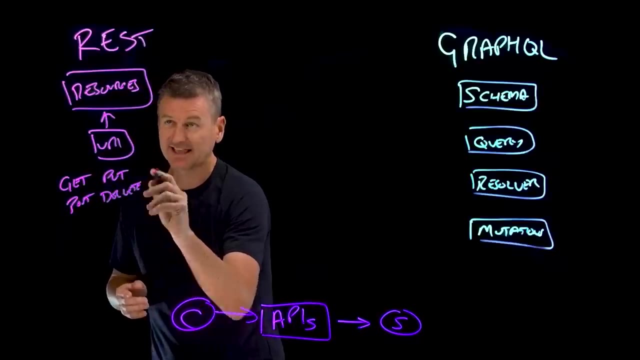 URI So it identifies. it's a uniform resource identifier and a client can request a response using an HTTP method. So the methods that we can use are get, put, post and delete, And that gets us access to those resources, And then the server responds with a. 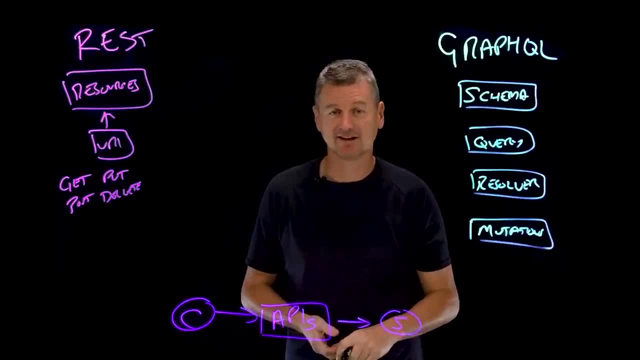 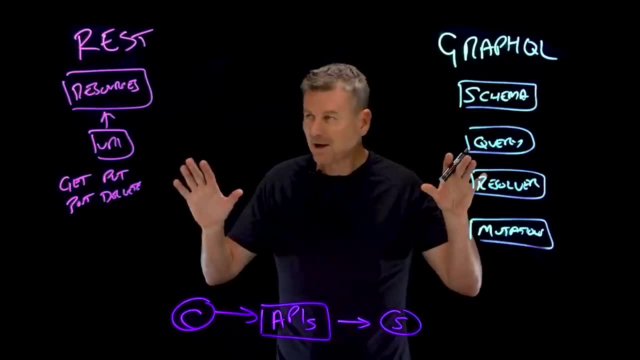 representation of the resource in a format like JSON or XML. Now, REST also allows clients to filter, sort and paginate the data using query parameters. So if we're going to do this in a different way, we're going to use a different type of 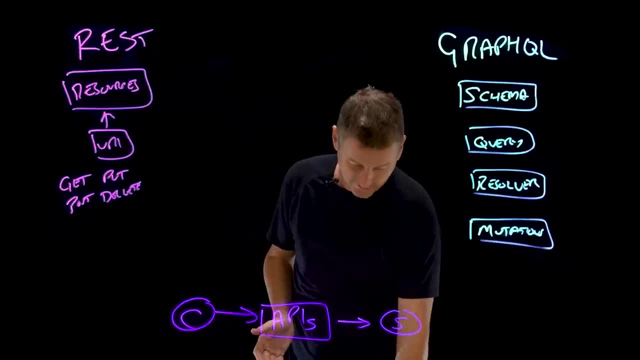 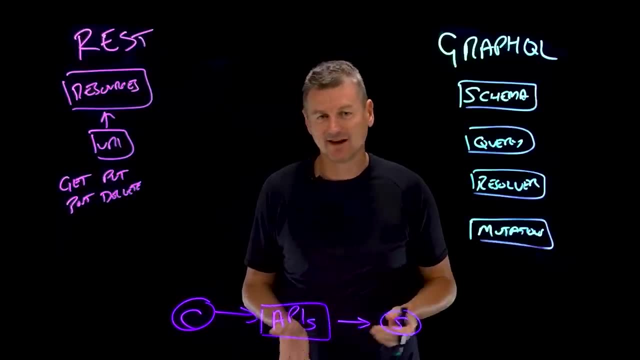 application. So how are GraphQL and REST similar? Well, both are used to, as I've mentioned, build APIs that allow different applications to communicate with each other over the Internet. Both also have a commonality in that they use frameworks and libraries to handle all of the 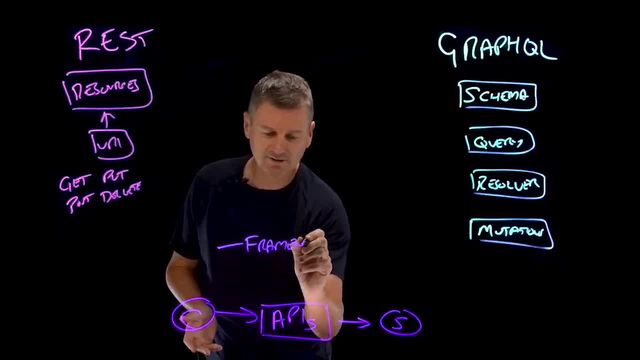 pesky network details, So we don't have to worry about them. And then also both operate over HTTP, although it is worth pointing out that GraphQL is protocol-agnostic, So that's one of the things that we're going to be looking at. 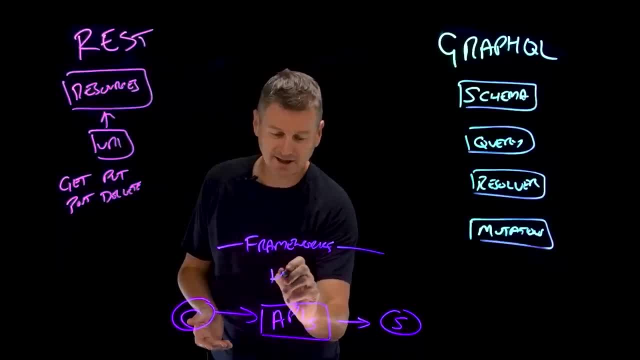 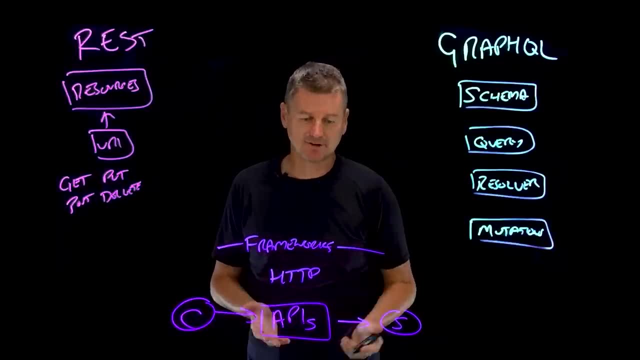 in the future. So let's take a look at some other applications. So let's take a look at some other applications. So let's take a look at some other applications. GraphQL is protocol-agnostic. GraphQL is protocol-agnostic Also. both can handle requests and 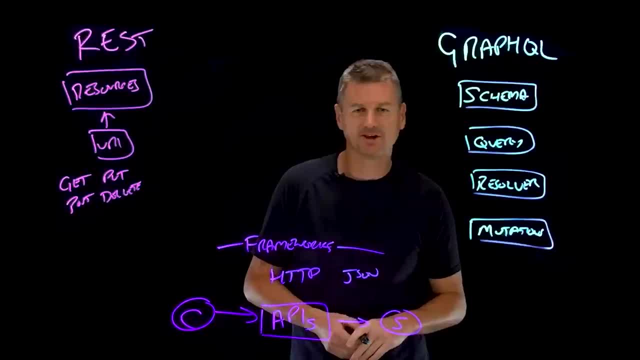 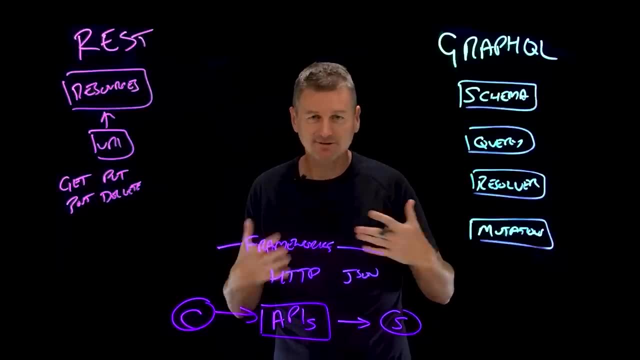 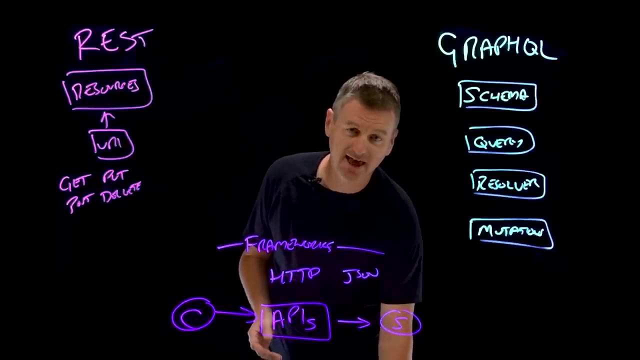 responses using JSON or the JavaScript object notation. But there are several key differences between the two technologies that make them better suited for different use cases. But there are several key differences between the two technologies that make them better suited for different use cases. When requesting data from a 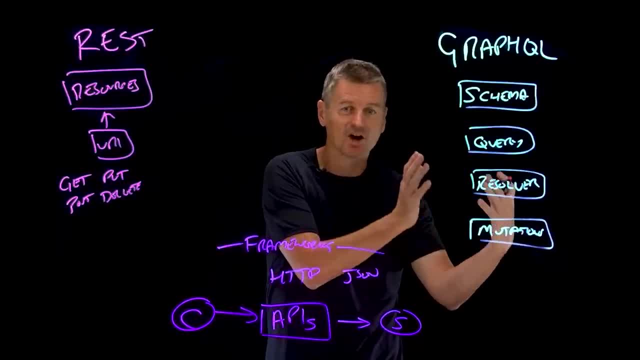 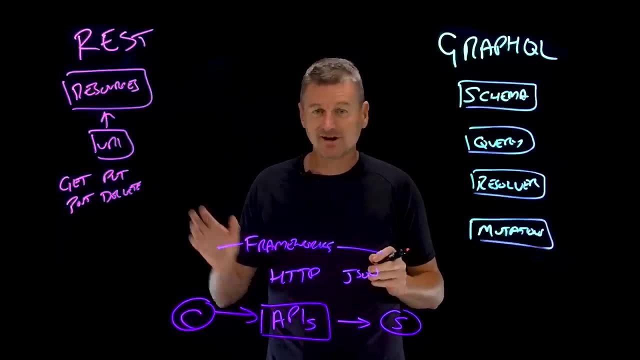 specific end point, a REST API returns the full dataset for that resource, whereas, in contrast, GraphQL is a query language specification. instead of tools that allow clients to BRLjis interact with a single endpoint, REST APIs often require multiple requests to fetch related data, while GraphQL can fetch. 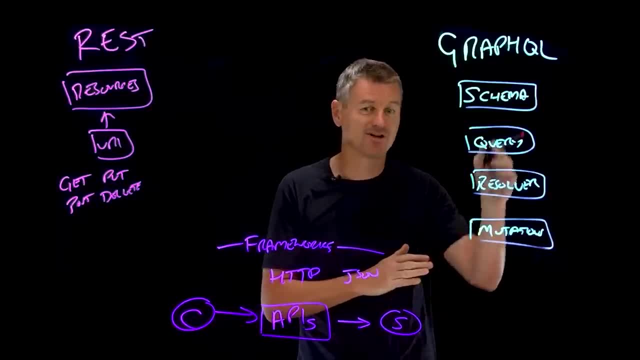 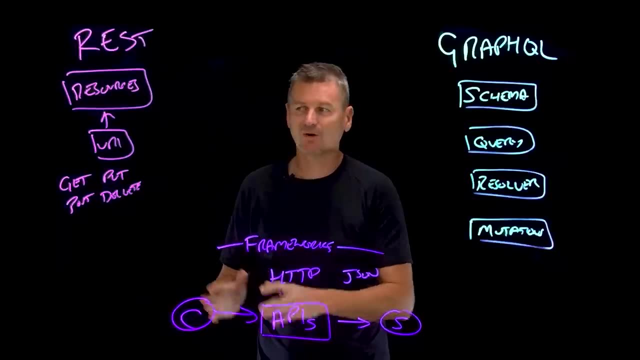 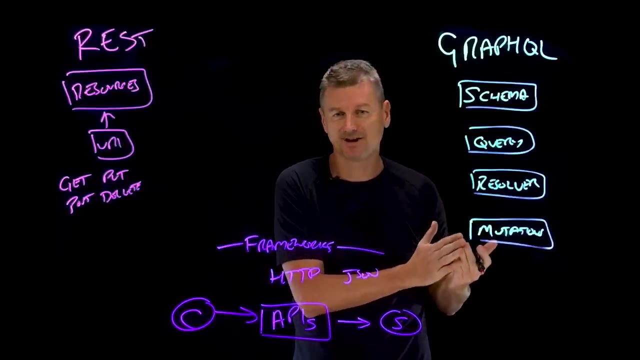 all the data in a single request using a complex query that follows the schema, So clients get what they request with no over-fetching. Now, REST APIs are already very familiar to many developers, so people know how to use them. GraphQL may represent a bit of a learning curve for some. 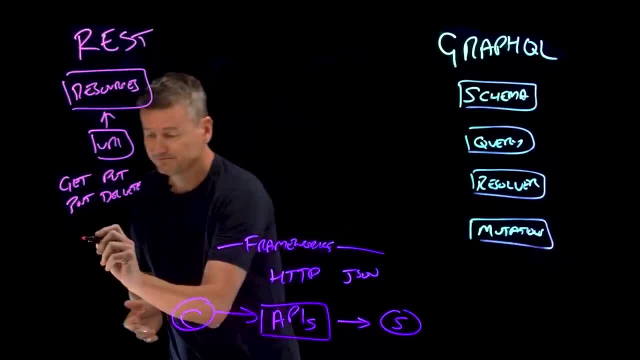 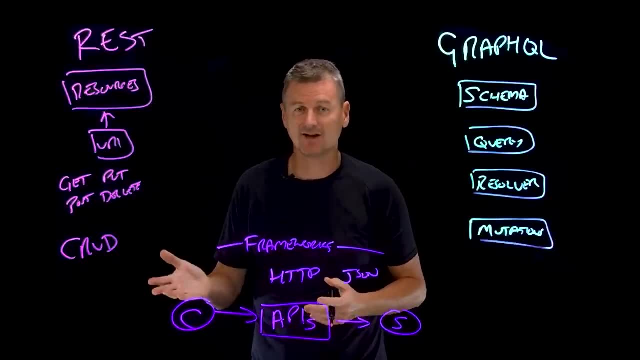 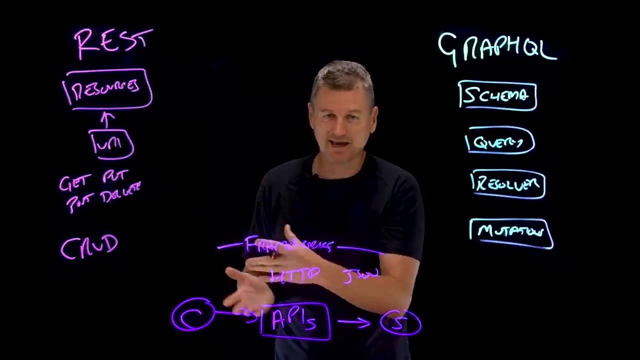 REST APIs are well-suited for applications that require simple CRUD-like operations. So, for example, an e-commerce website might use a REST API to allow customers to browse products, add items to their cart and complete orders. In that case, the API would use the HTTP methods we talked about: get, put, post and delete. 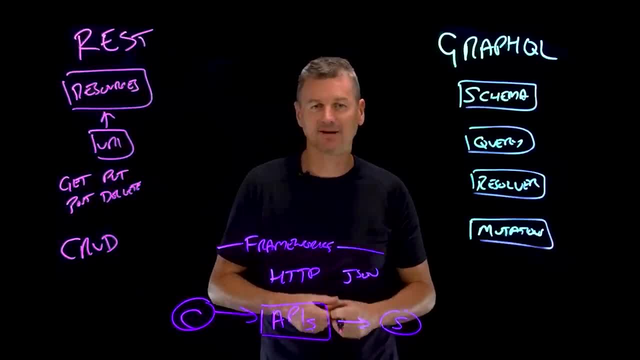 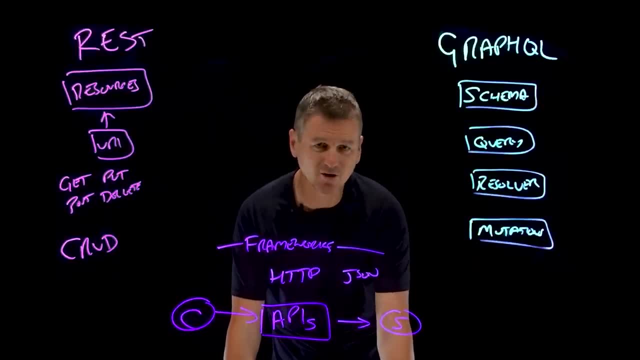 to manipulate the data, like the products, the orders and the customer information. Now, on the other hand, GraphQL is better suited for applications that require multiple requests. GraphQL is better suited for applications that require well a bit more complex data requests. 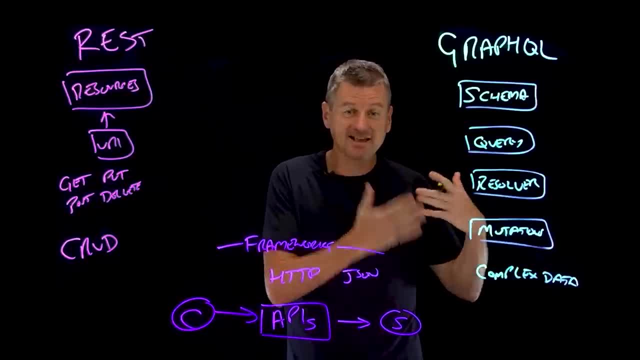 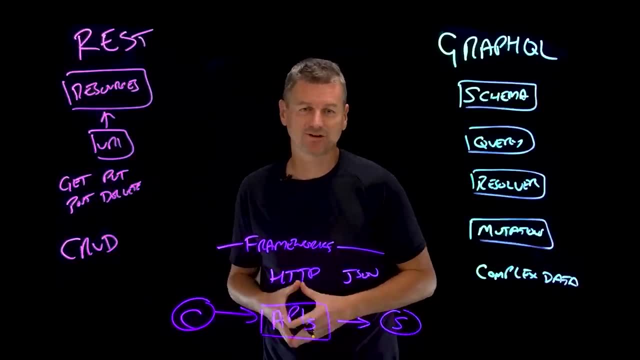 And what I mean by that is where we have examples of many sort of nested fields or multiple data sources that we need to pull from. So if we think about a company that provides a suite of financial planning tools for its clients, those tools might require data from multiple sources. 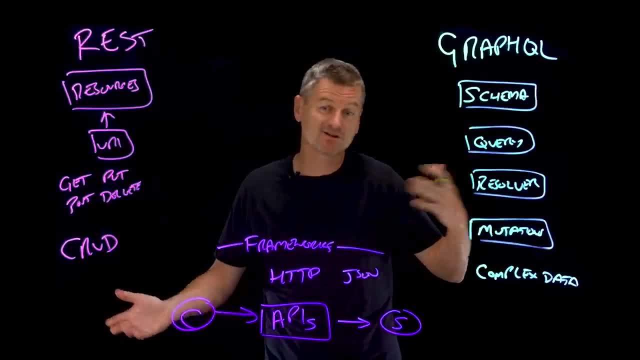 So they might need to go to bank transactions, investment portfolios and credit scores, And with GraphQL the company can build a schema. That's a great way to build a schema. That's a great way to build a schema. That's a great way to build a schema. 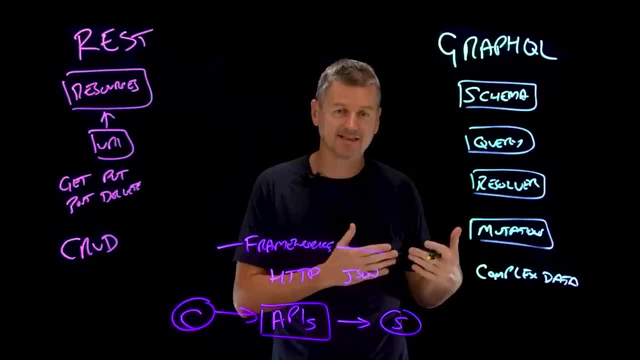 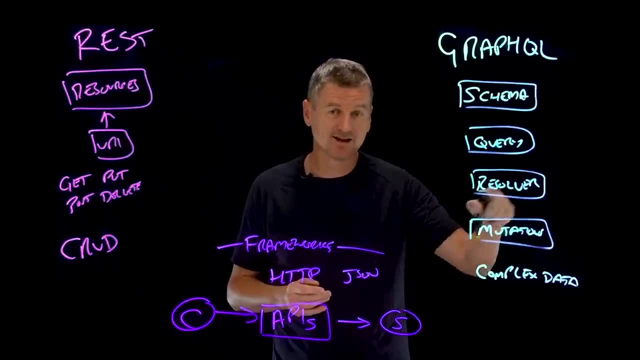 It's a single API endpoint that allows clients to query all of the data in a single request, So clients simply specify exactly the data that they need and the server would use a set of resolvers to fetch the necessary data from each source and assemble it into a response.